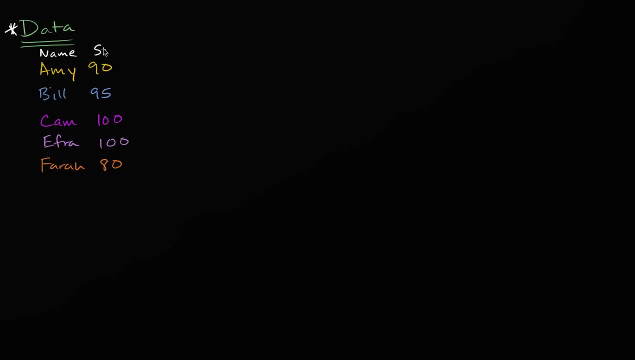 where you have the name, let me, and then you have the score. so you have your name, column, and then you have your score, column, and I could construct it as a table so it clearly looks like a table, like that: 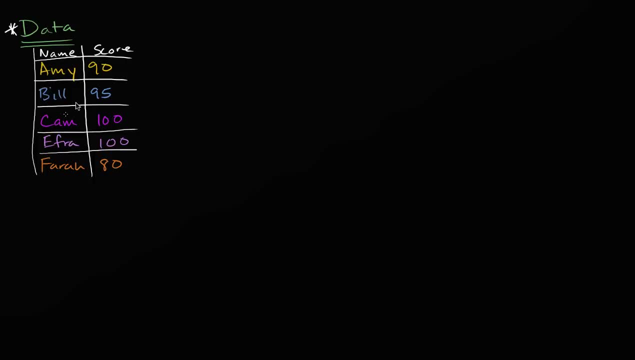 That's one way, one very common way, of representing data just like that. That's actually how most traditional databases record data in tables like this, But you could also do it in other ways, So you could record it as a oftentimes called a bar graph, or sometimes a histogram. 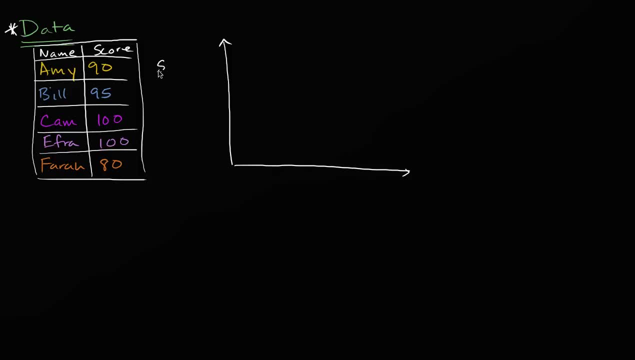 So you could put score on the vertical axis here and then you could have your names over here and let's see the scores. let's see, maybe I'll make this in, let's make this a 50, actually, let me just mark them off. 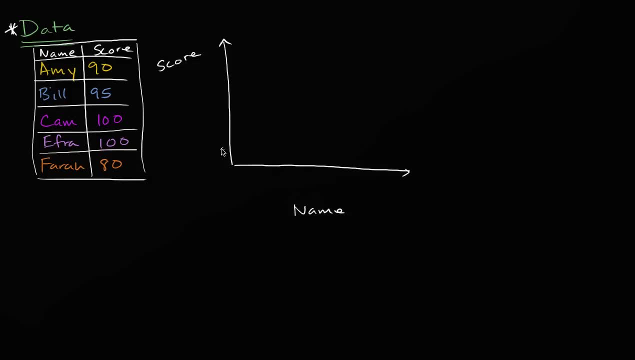 so this is 10,, 20,, 30,- no, that's too big- 10,, 20,, 30,, 40,, 50,, 60,, 70,, 80,, 90, so that's, and then 100, so that's 100,. 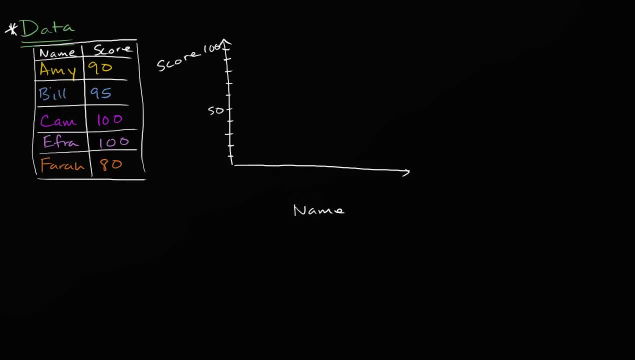 one, two, three, four, five. that would be 50 right over there, And then you could go person by person. so Amy, Amy got a 90 on the exams, so the bar will go up to 90.. So that is Amy, and then you have Bill. 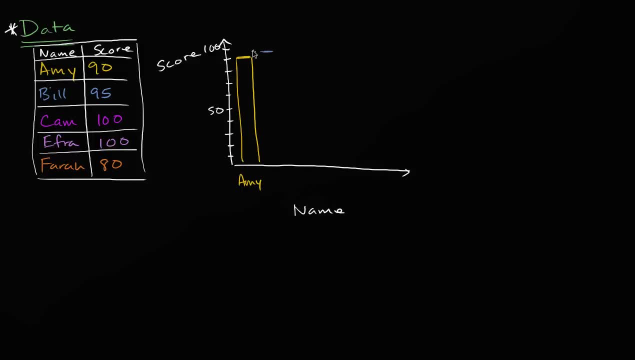 got a 95, so it's gonna be between 90 and 100, so it's gonna be right over there. Bill got a 95, and so it would look like this: Bill. so that is Bill. And then you have Cam, who got a 100 on the exam. 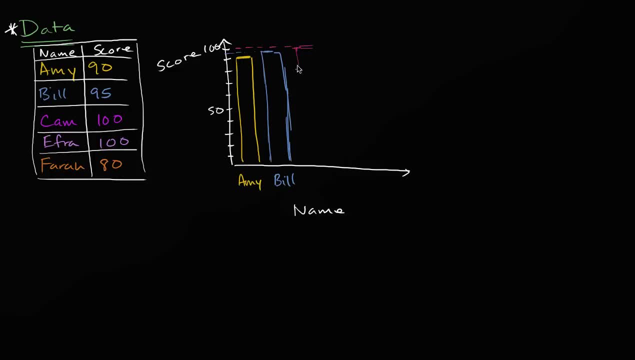 so make sure, obviously I'm hand drawing it so it's not as it's not as precise as if I were to do it on a computer. So this right over there, that is Cam's score. Efra got the same score as Cam. 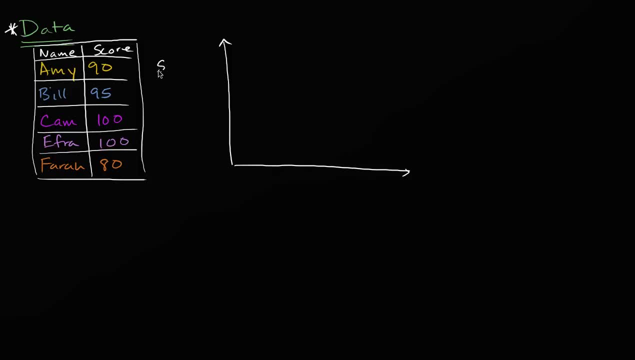 So you could put score on the vertical axis here and then you could have your names over here and let's see the scores. let's see, maybe I'll make this in, let's make this a 50, actually, let me just mark them off. 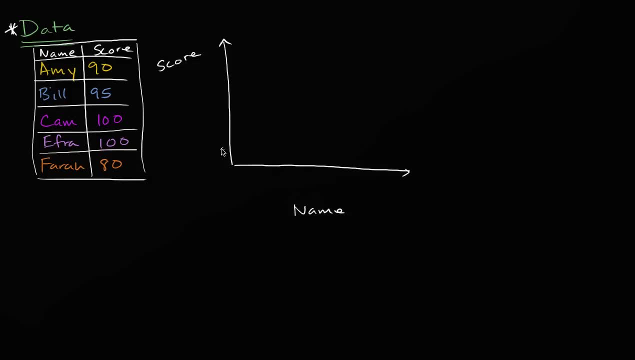 so this is 10,, 20,, 30,- no, that's too big- 10,, 20,, 30,, 40,, 50,, 60,, 70,, 80,, 90, so that's, and then 100, so that's 100,. 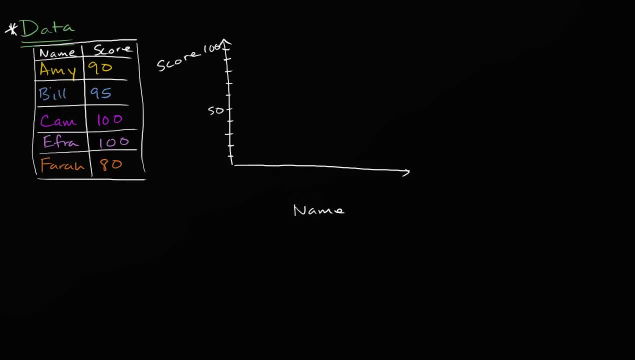 one, two, three, four, five. that would be 50 right over there, And then you could go person by person. so Amy, Amy got a 90 on the exams, so the bar will go up to 90.. So that is Amy, and then you have Bill. 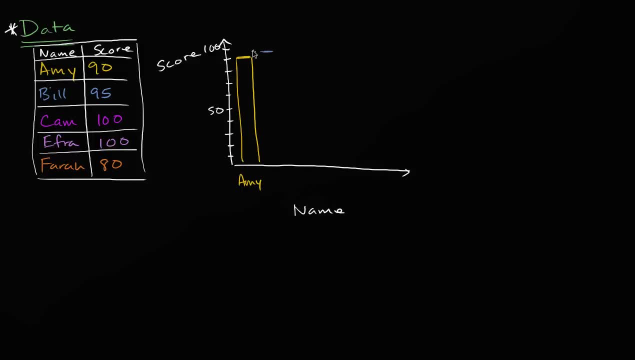 got a 95, so it's gonna be between 90 and 100, so it's gonna be right over there. Bill got a 95, and so it would look like this: Bill. so that is Bill. And then you have Cam, who got a 100 on the exam. 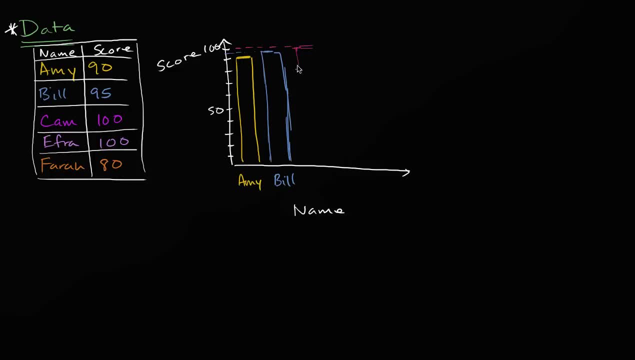 so make sure, obviously I'm hand drawing it so it's not as it's not as precise as if I were to do it on a computer. So this right over there, that is Cam's score. Efra got the same score as Cam. 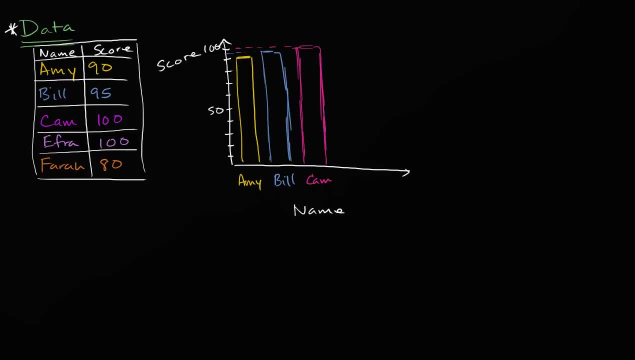 so her score is going to be- let me do that in the color, in Efra's color. That's Efra's score right now. there she also got 100.. So Efra, Efra and then finally Farah got an 80,. 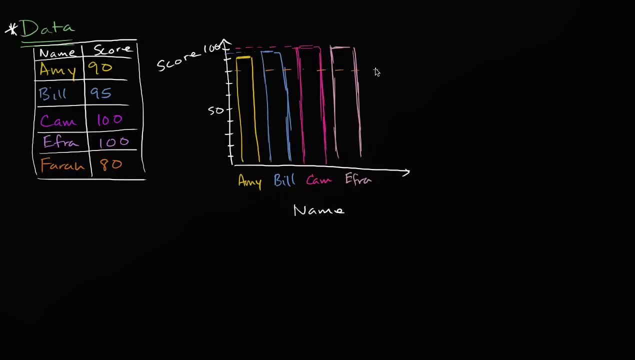 so 60,, 70,, 80, so Farah got got an 80,. so this is Farah's score right over here. So this is another way of representing the data, And here we see it in visual form. 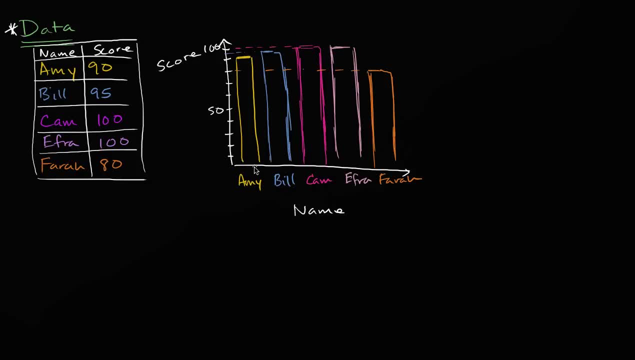 but it has the same information. You can look up someone's name and then figure out their score. Amy scored a 90,, Bill scored a 95,, Cam scored 100,, Efra also scored 100,, Farah scored an 80, and there's even other ways. 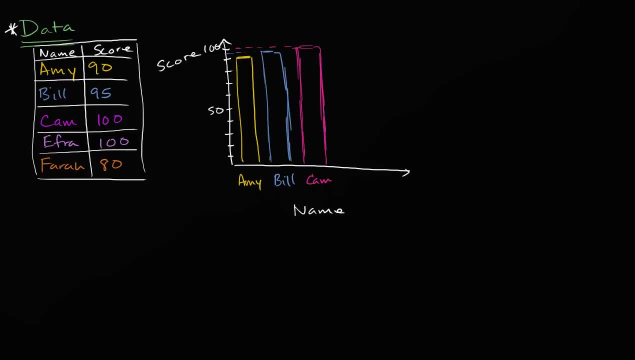 so her score is going to be- let me do that in the color, in Efra's color. That's Efra's score right now. there she also got 100.. So Efra, Efra and then finally Farah got an 80,. 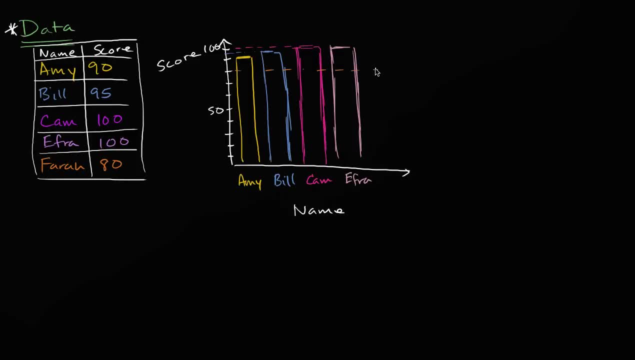 so 60,, 70,, 80, so Farah got got an 80,. so this is Farah's score right over here. So this is another way of representing the data, And here we see it in visual form, but it has the same information. 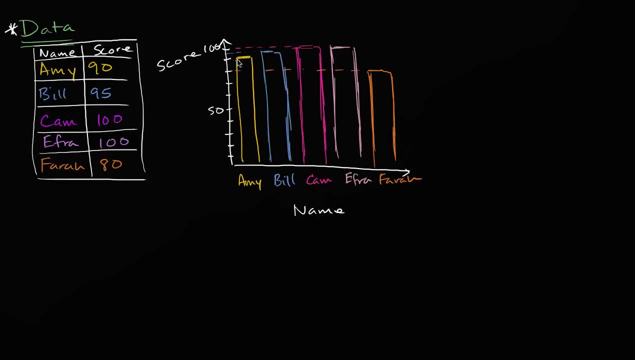 You can look up someone's name and then figure out their score. Amy scored a 90,, Bill scored a 95,, Cam scored a 100,, Efra also scored a 100,, Farah scored an 80, and there's even other ways. 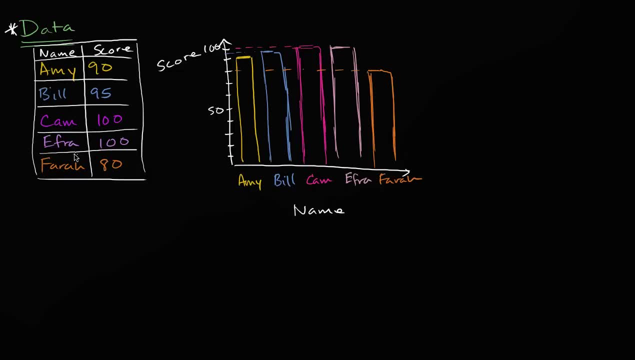 you can have some of this information. In fact, sometimes you might not even know their names, and so then it would be less information, but it might just be a list of scores. The professor might say: hey, here are the five scores. 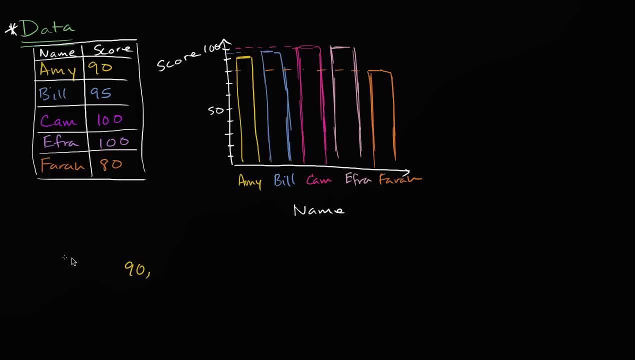 that people got on the exam and they would list 90,, 95,, 95,, 100, 100, 100, and 80. Now, if it was listed, if this was all of the data you got, this would be less information than the data. 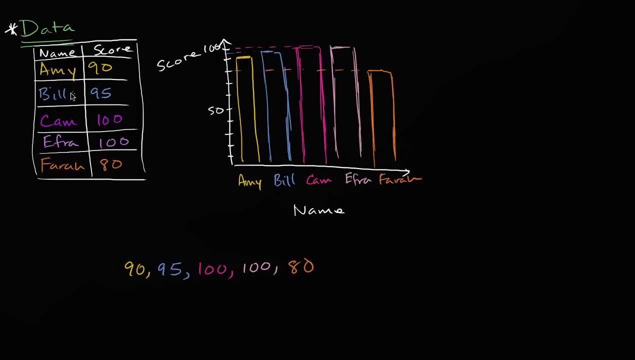 that's in this bar graph or this histogram or the data that's given in this table right over here, Because here not only do we know the scores, but we know who got what score. Here we only know the list of scores. 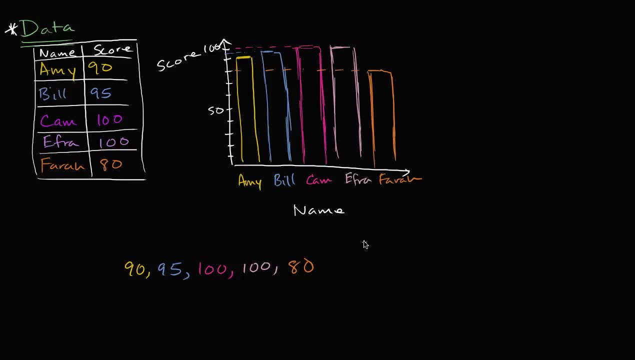 But there's even other ways, and this is not an exhaustive video of all of the different ways you can represent data. You could also represent data by looking at the frequency of scores, So the frequency of scores right over here. So instead of writing the people, you could write the scores. 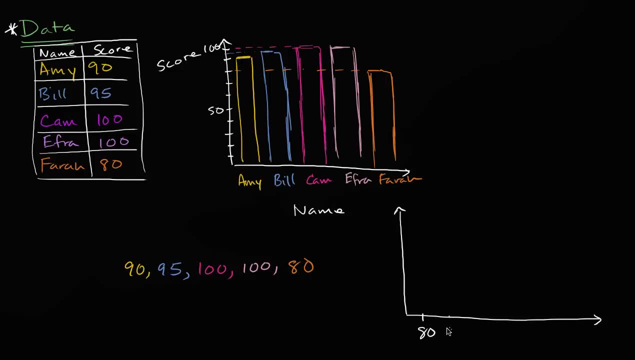 So let's see, you could say this is 80,, 85,, 90,, 95, and 100, and then you could record the frequency that people got these scores. So how many times do you have a score of an 80?? 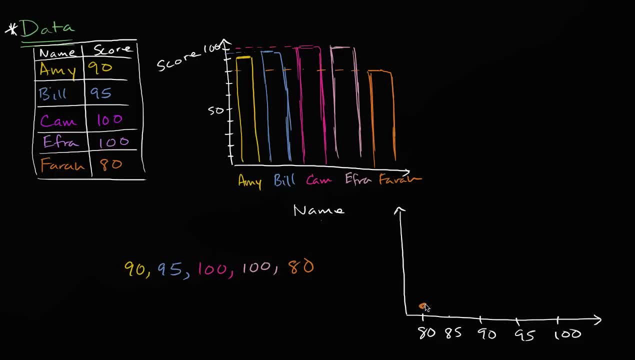 Well, Farah is the only person with a score of 80, so you put one data point there. No one got an 85,. one person got a 90, so you put a data point there. One person got a 95, so you could put that data point. 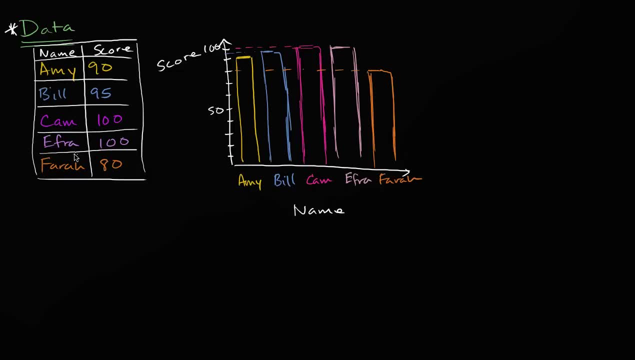 you can have some of this information. In fact, sometimes you might not even know their names, and so then it would be less information, but it might just be a list of scores. The professor might say: hey, here are the five scores. 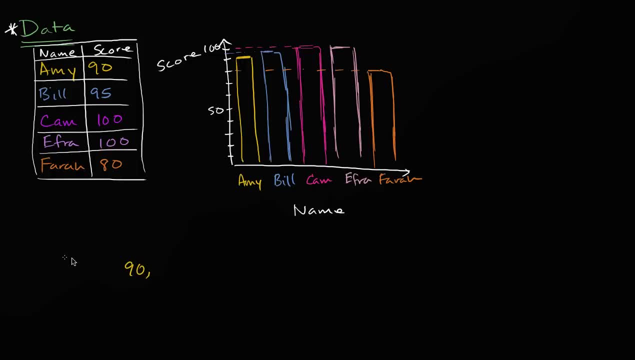 that were that people got on the exam and they would list 90,, 95,, 95,, 100,, 100,, 100, and 80. Now, if it was listed in, if this was all of the data? 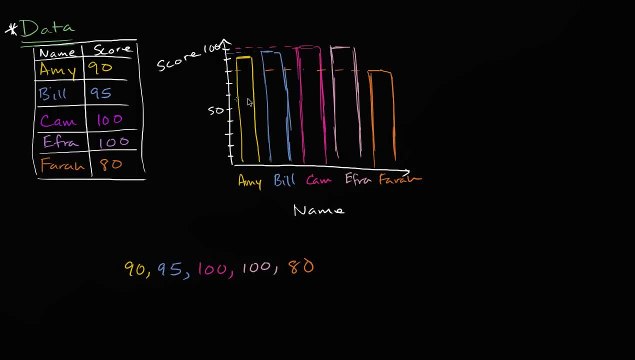 you got. this would be less information than the data that's in this bar graph or this histogram or the histogram or the data that's given in this table right over here, Because here not only do we know the scores, but we know who got what score. 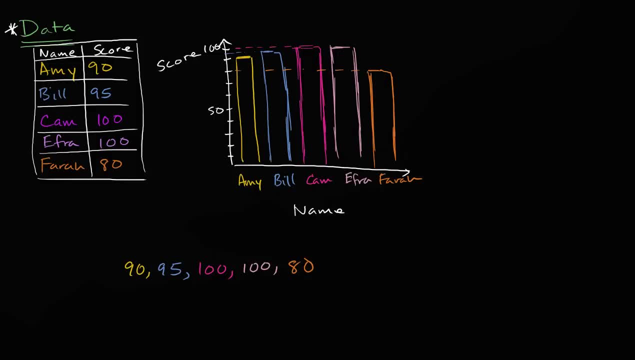 Here we only know the list of scores, But there's even other ways and this is not an exhaustive video of all of the different ways you can represent data. You could also represent data by looking at the frequency of scores. So the frequency of scores right over here. 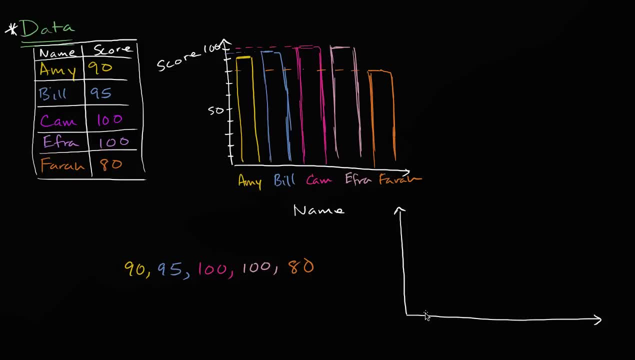 So instead of writing the people, you could write the scores. So let's see, you could say this is 80,, 85,, 90,, 95, and 100. And then you could record the frequency that people got these scores. 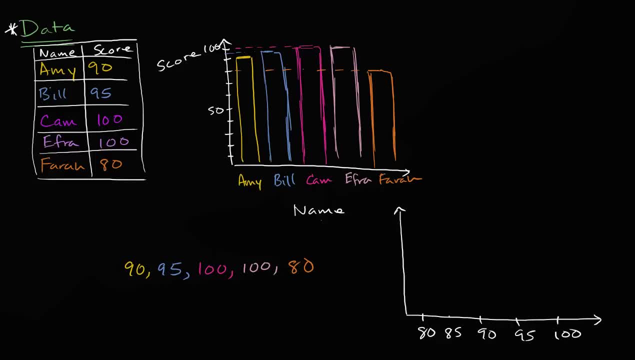 So how many times do you have a score of an 80?? Well, Farah is the only person with a score of 80, so you put one data point there. No one got an 85,. one person got a 90,. 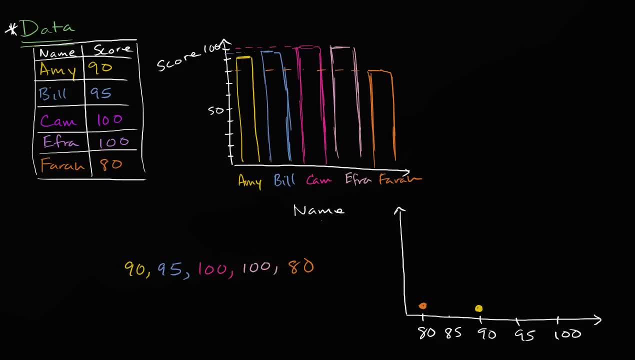 so you put a data point there. One person got a 95, so you could put that data point right over there. And then two people got a 100. So this is one and two. Let's see the other 100 is in this color. 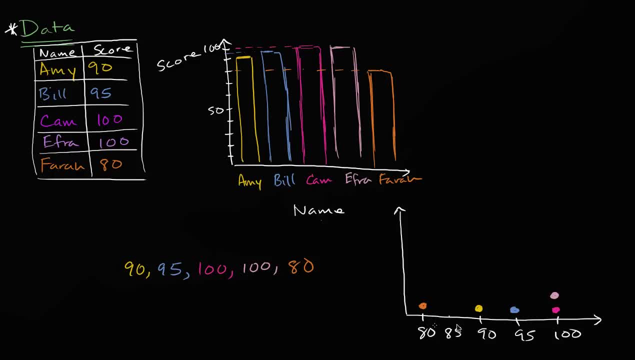 so I'll just do it in the color. You wouldn't necessarily have to color code it like this. So this is another way to represent, and this is, you know, this axis. you could just view this as the number. So this tells you how many 80s there were. 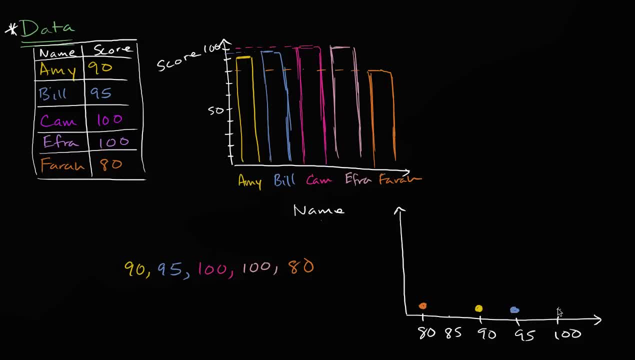 right over there and then two people got 100. So this is one and two. Let's see the other 100 is in this color, So I'll just do it in the color. You wouldn't necessarily have to color code it like this. 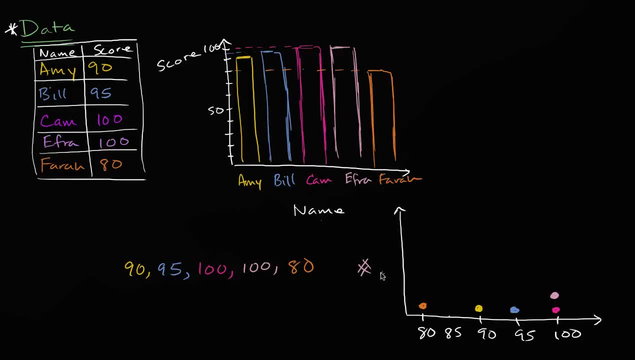 So this is another way to represent And this is on this axis. you could just view this as the number. So this tells you how many 80s there were, How many 90s there are, How many 95s and how many 100s. 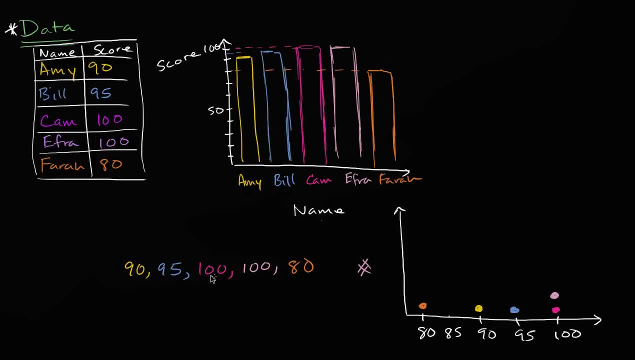 So this right over here has the same data as this list of numbers. It's just another way of looking at it. Once you have your data arranged in any of these ways, we can start to ask interesting questions. We can ask ourselves things like: 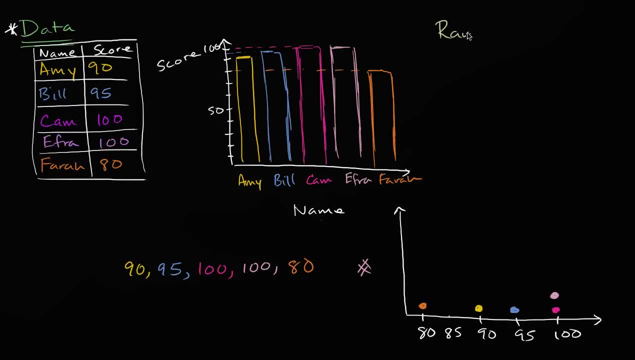 well, what is the range of data? What is the range in the data? And the range is just the spread between the lowest point and the highest point. So the range in this data is gonna be the difference between the highest score, and the highest scores are 100,. 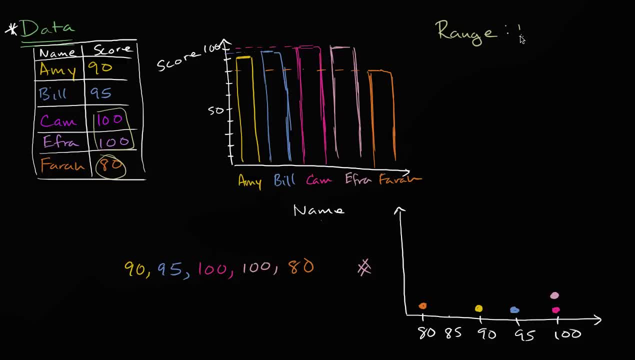 and the lowest score an 80. So the range is going to be the difference between the max minus the min, The maximum score minus the minimum score, So it's gonna be 100 minus 80 is equal to 20.. So that gives you a sense of things. 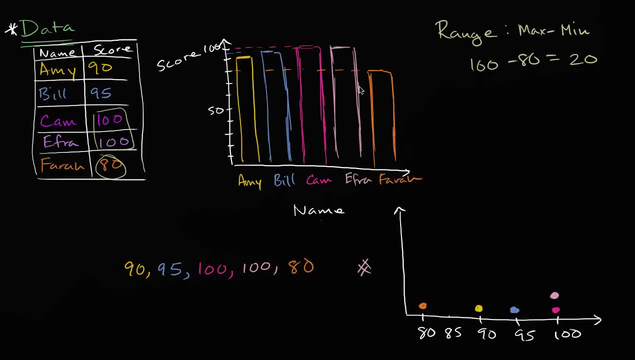 It kind of gives you a sense of spread. You could also ask yourself: well, how many people scored below 100?? These are just interesting questions Below 100. And you can actually answer that question. well, actually, you could have answered. 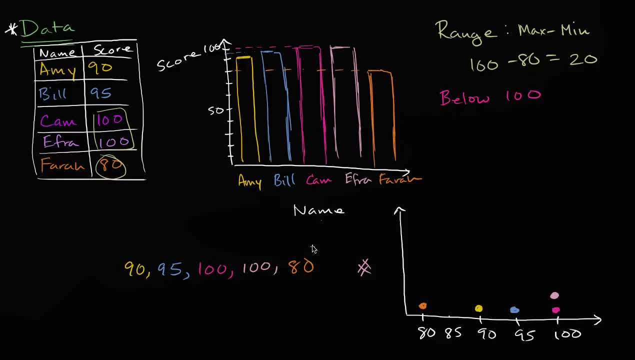 either of these questions, with any of these different ways of looking at the data. If you say how many people scored below 100, well, one, two, three. How many people scored below 100? Well, 100 is up here. so it's gonna be one, two, three. 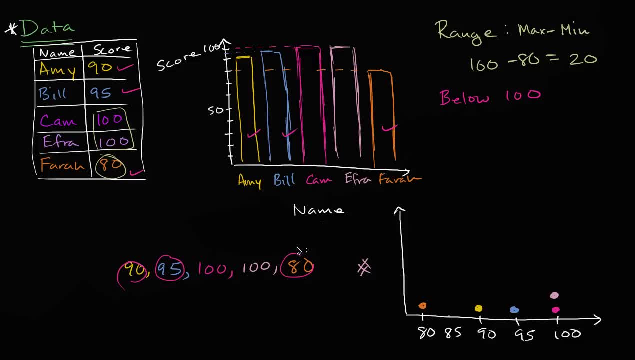 How many people scored below 100? One, two, three. How many people scored below 100? One, two, three. And so, any way you look at it, you would have gotten three. And you could also ask yourself: 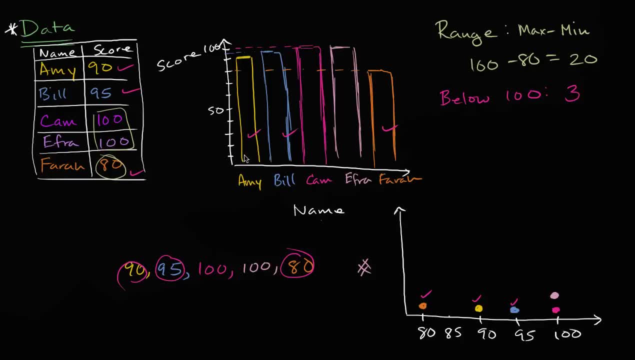 what is the most frequent score? So most frequent, Most frequent, Frequent, And once again, you could answer that question with any of these ways of representing this data. You could look at our original table and you say, look, there's only 190,, 195,, 180,, there's two hundreds. 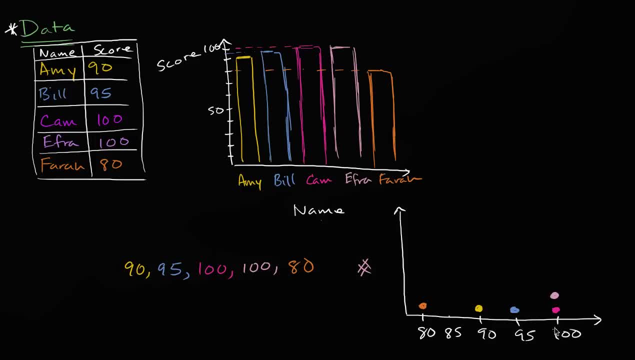 how many 90s there are, how many 95s and how many 100s. So this right over here has the same data as this list of numbers. It's just another way of looking at it, And once you have your data arranged in any of these ways, 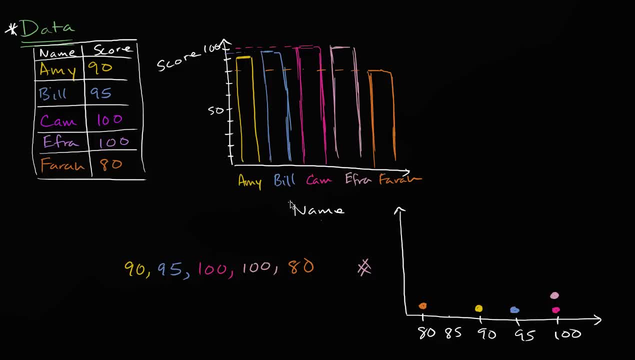 we can start to ask interesting questions. We can ask ourselves things like: well, what is the range of data? What is the range in the data? And the range is just the spread between the lowest point and the highest point, So the range in this data is gonna be the difference. 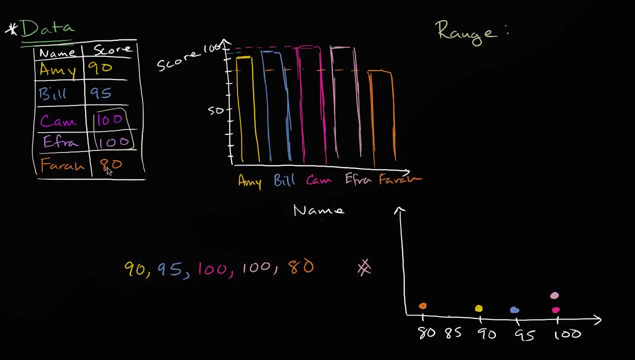 between the highest score and the highest scores are 100, and the lowest score an 80. So the range is going to be the difference between the max minus the min. The maximum score minus the minimum score- So it's gonna be 100 minus 80- is equal to 20.. 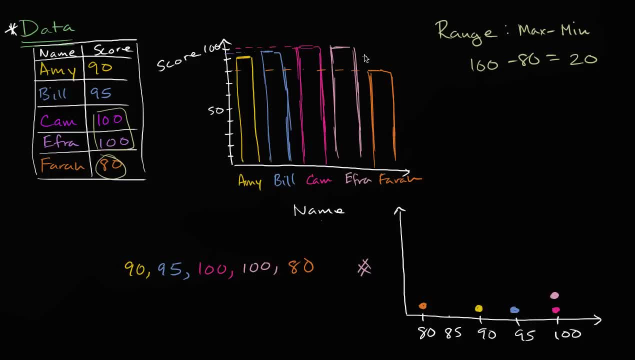 So that gives you a sense of things. It kind of gives you a sense of spread. You could also ask yourself: well, how many people scored below 100?- And these are just interesting questions- Below 100. And you can actually answer that question. 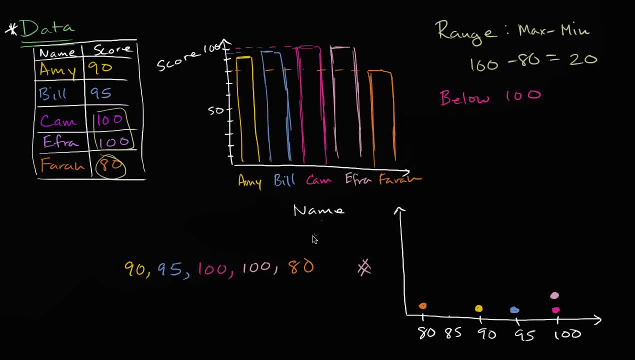 well, actually, you could have answered either of these questions With any of these different ways of looking at the data. If you say how many people scored below 100? Well, one, two, three, How many people scored below 100?? 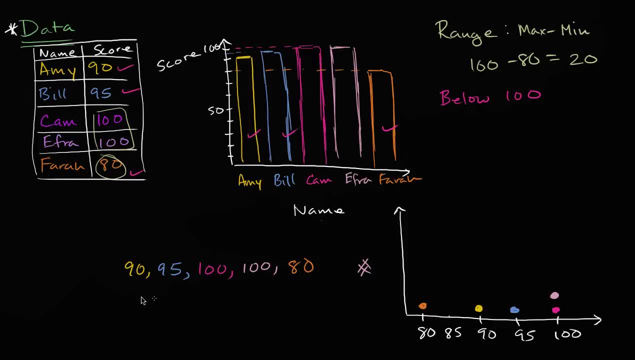 Well, 100 is up here, so it's gonna be one, two, three. How many people scored below 100? One, two, three. How many people scored below 100? One, two, three. And so, any way you look at it, 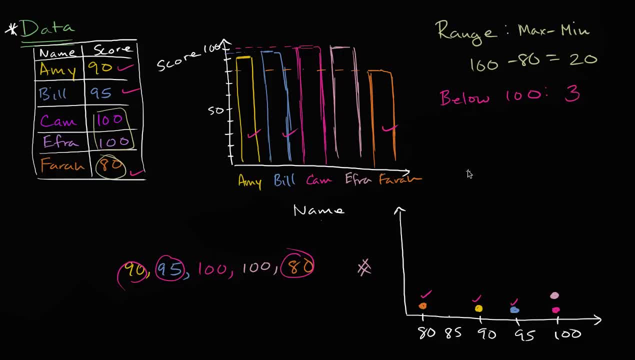 you would have gotten three And you could also ask yourself: what is the most frequent score? So, most frequent, Most frequent? And once again, you could answer that question. with any of these ways of representing this data, You could look at our original table. 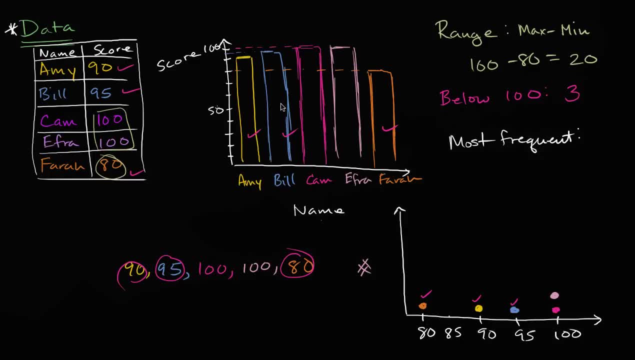 and you say: look, there's only 190,, 195,, 180.. There's two hundreds. So you'd say: look, the most frequent score is 100.. You'd see that over here too, You actually have two hundreds. 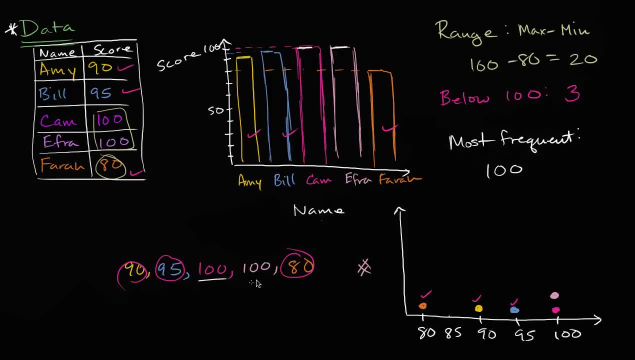 There's only one of each of the other scores. Here you also see the two hundreds And here is probably the clearest. if you're looking at frequency, Sometimes this might be called a frequency plot, Sometimes it's called a. well, the, the, the, the, the, sometimes the official. 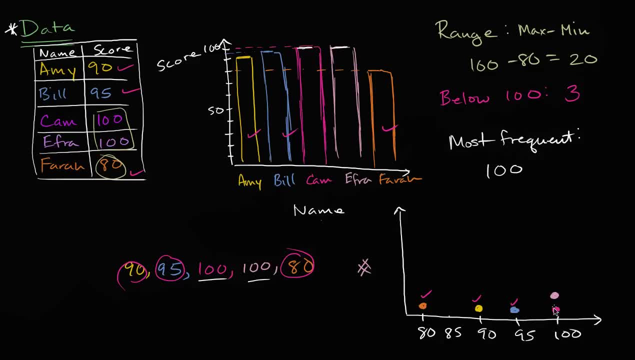 well, it's often called a frequency plot And you see here the most frequent one is the one that has the most dots on it, which is 100.. So, anyway, that's just a very high level overview of how you can look at data.